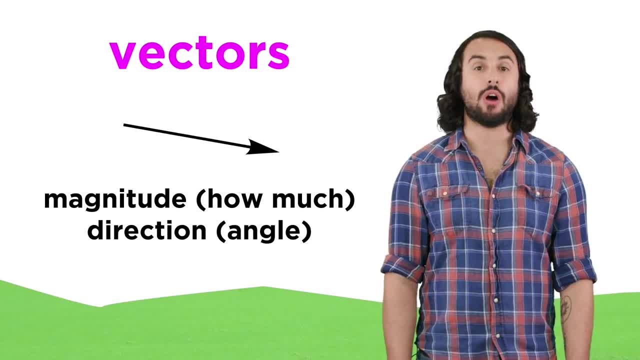 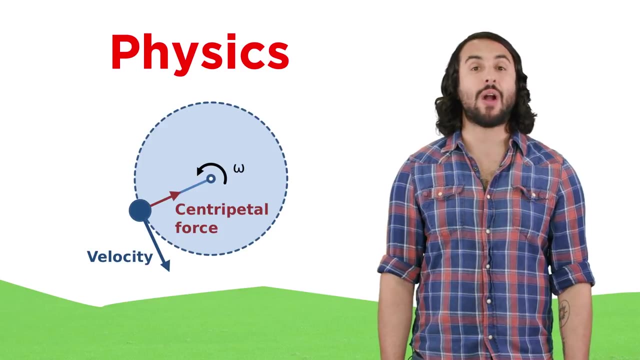 The length of the vector tells us the magnitude, so a longer vector means a greater magnitude, and the direction the arrow points relative to some axes tells us the direction of the vector. Vectors are of tremendous importance in physics because they describe things like forces that 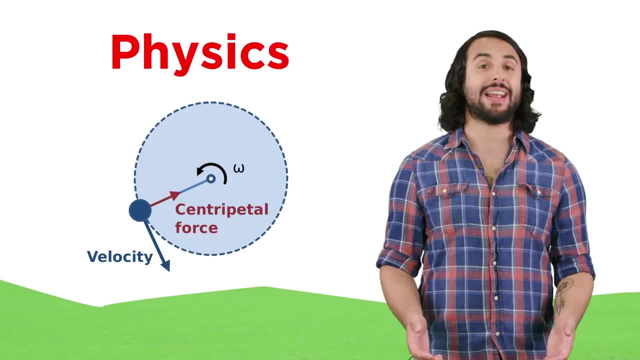 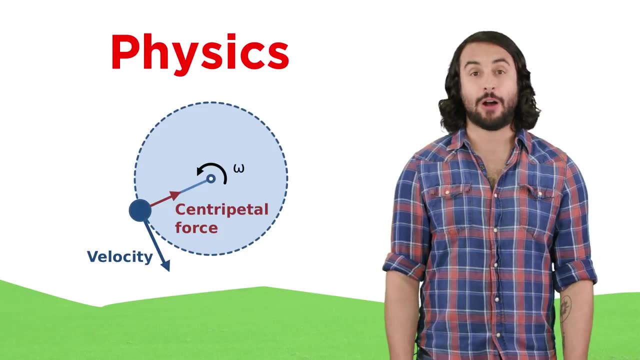 cause the three-dimensional motion of objects. You can check out some of the things we can do with vectors after this by checking out my classical physics series, But for now, let's go ahead and learn all the things we need to know about vectors in. 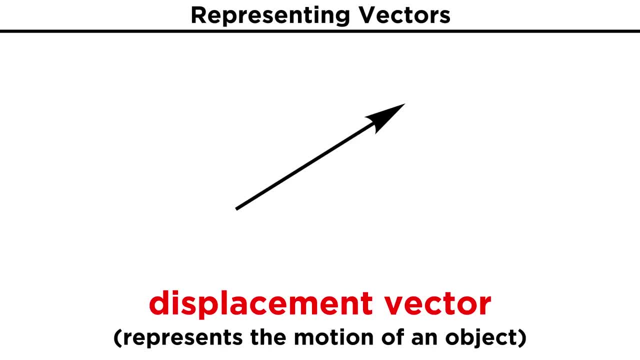 order to do more math, Many vectors are simply displacement vectors, denoting how far an object is. If such a vector connects two points like A and B, we can call this vector AB, with a little arrow over it. That's one way to represent a vector. 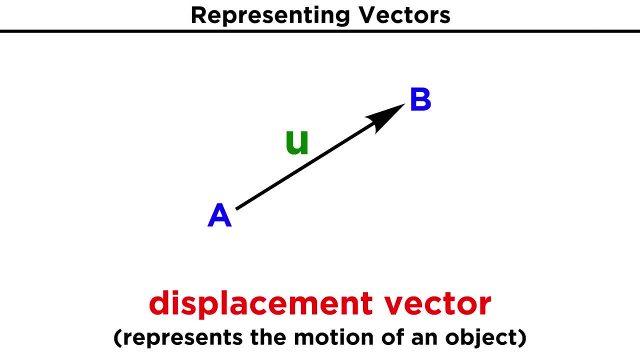 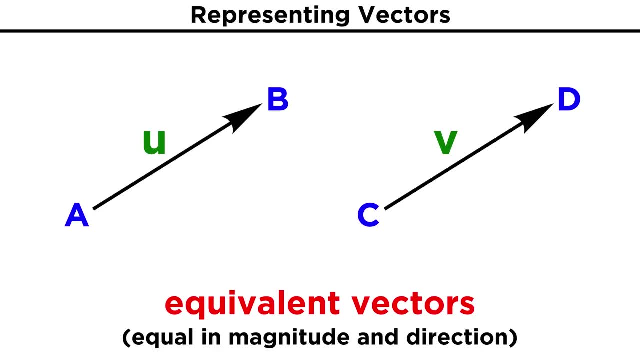 We can also just refer to a vector with a letter like U. Different vectors with the same magnitude and direction are called equivalent vectors. But of course vectors can have different magnitudes and directions and we can manipulate and combine vectors in various ways. 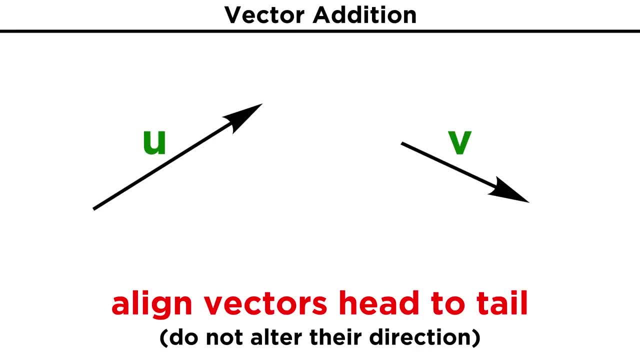 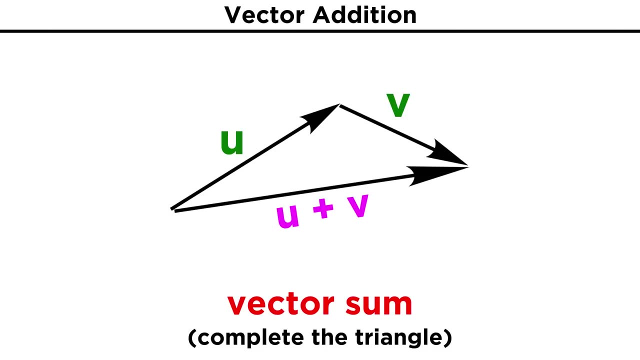 First, there is vector addition. If we have vector U and vector V and we place them head to tail, with V starting where U ends, being very careful not to alter the direction of either vector, then the sum of these vectors, or U plus V, will simply go from the start of U to the end of V, forming. 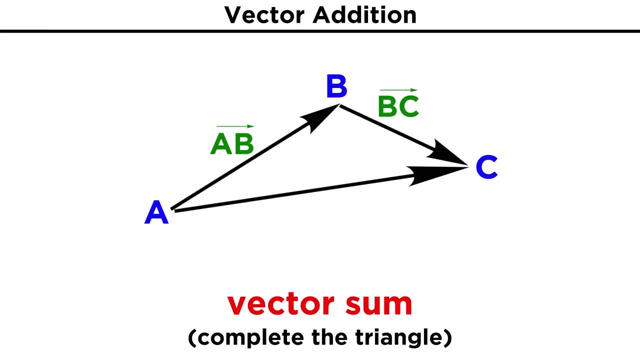 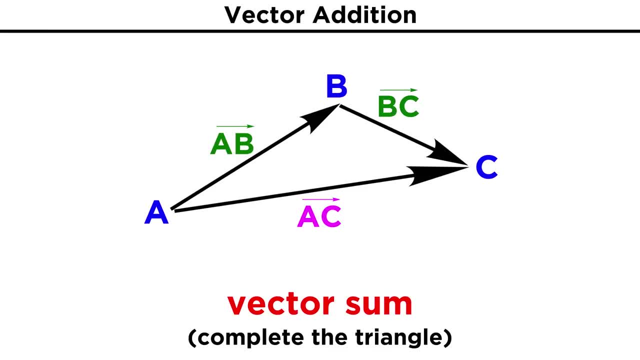 If these vectors were AB and BC, their sum would be U plus V. If these vectors were ABC, their sum would be called AC, as it would connect A and C. We don't necessarily have to draw triangles, though. Let's say U and V start at the same point. 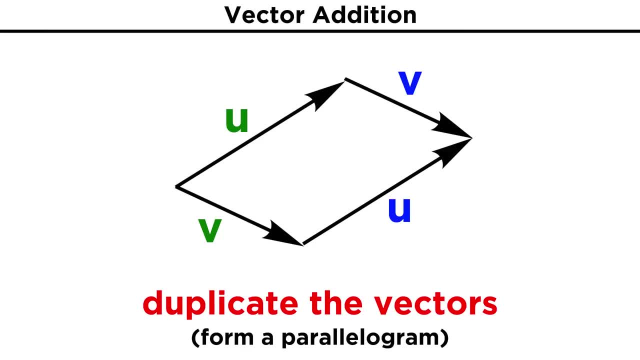 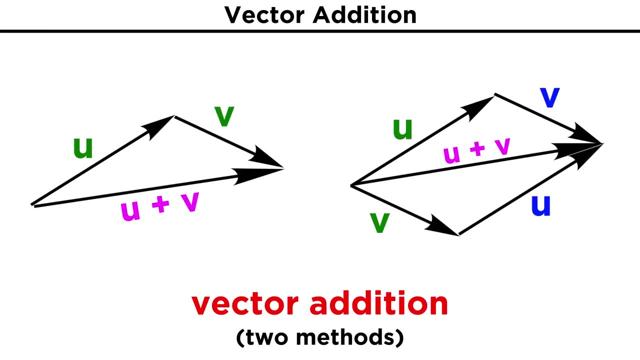 Let's duplicate U and V and move them so as to form a parallelogram like this. Now the sum of the two vectors, U plus V, can be represented as the diagonal of the parallelogram. So there are a number of ways to represent vector addition. 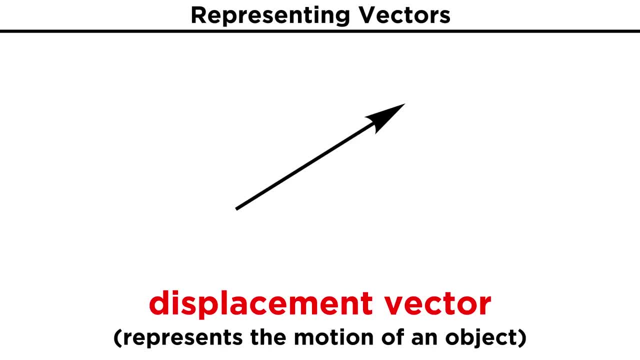 order to do more math, Many vectors are simply displacement vectors, denoting how far an object is. If such a vector connects two points like A and B, we can call this vector AB, with a little arrow over it. That's one way to represent a vector. 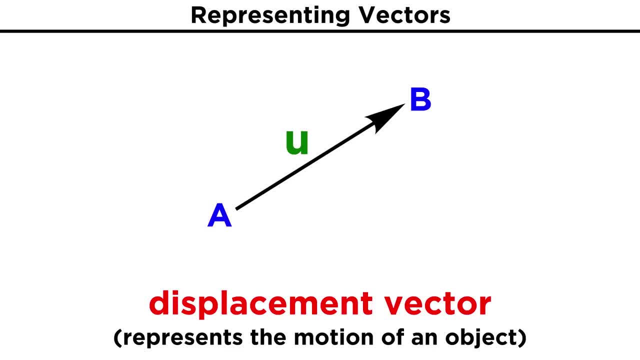 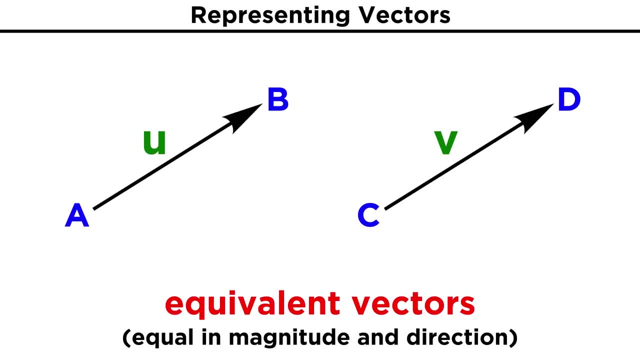 We can also just refer to a vector with a letter like U. Different vectors with the same magnitude and direction are called equivalent vectors. But of course vectors can have different magnitudes and directions and we can manipulate and combine vectors in various ways. 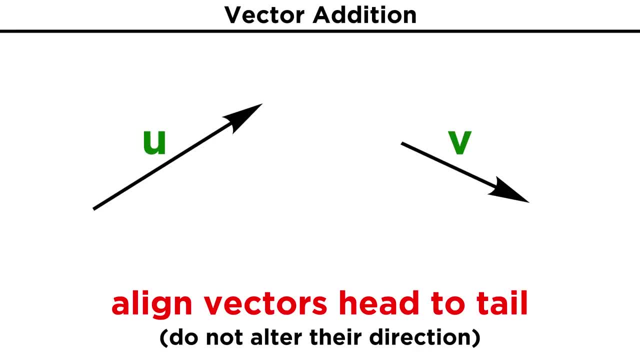 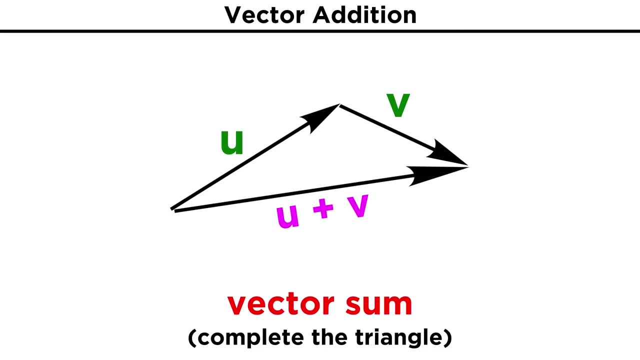 First, there is vector addition. If we have vector U and vector V and we place them head to tail, with V starting where U ends, being very careful not to alter the direction of either vector, then the sum of these vectors, or U plus V, will simply go from the start of U to the end of V, forming. 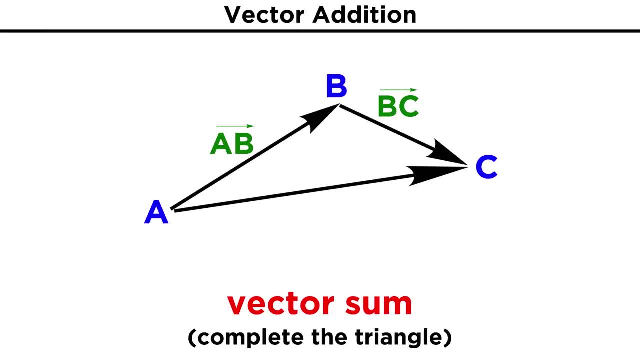 a triangle like so: If these vectors were AB and BC, their sum would be U plus V. If these vectors were AB and BC, their sum would be AB and BC. If these vectors were AB and BC, their sum would be AB and BC. 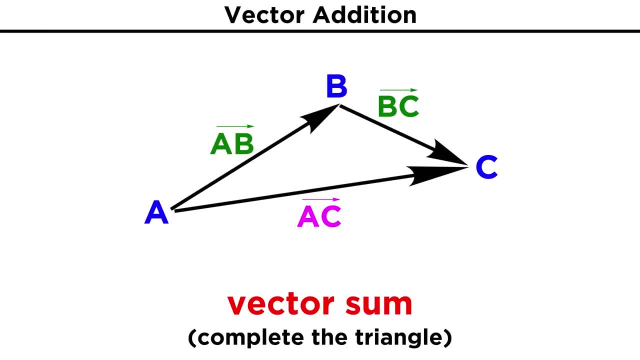 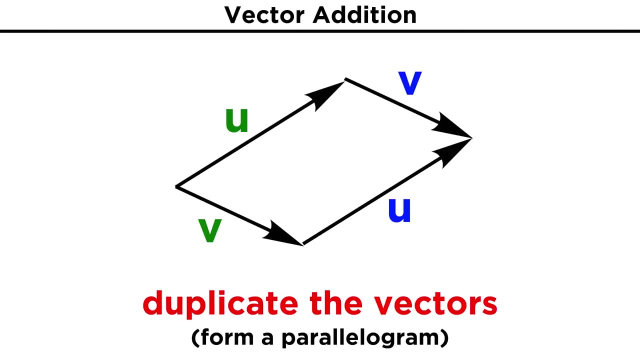 And if these vectors were AC and AC, their sum would be called AC, as it would connect A and C. We don't necessarily have to draw triangles, though. Let's say U and V start at the same point. Let's duplicate U and V and move them so as to form a parallelogram like this: 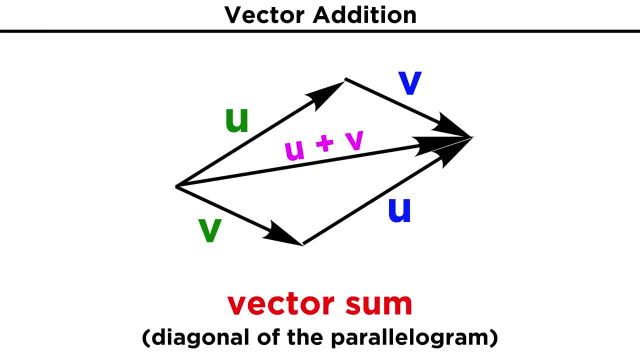 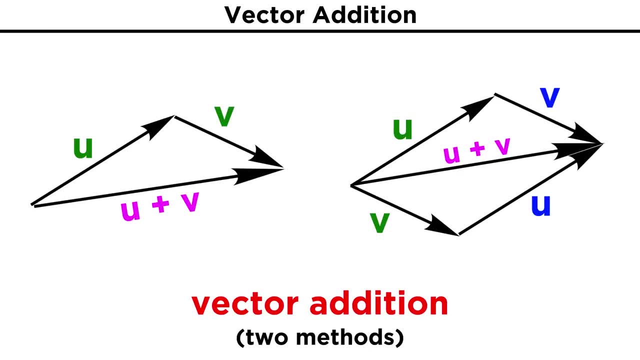 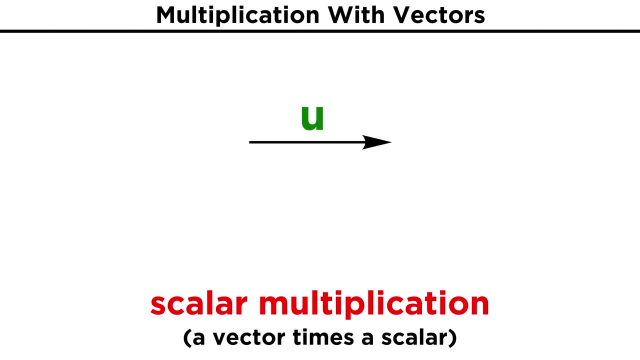 Now the sum of the two vectors U plus V can be represented as the diagonal of the parallelogram. So there are a number of ways to represent vector addition. represent vector addition geometrically. We can also perform multiplication with vectors. 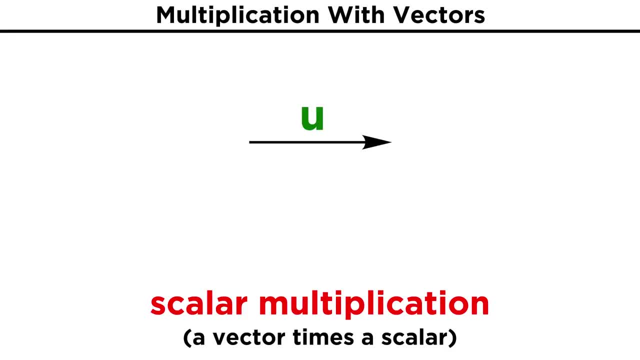 The simplest way to do this is called scalar multiplication. This is when a vector is multiplied by a scalar which is just a number. So if we have some vector u and we multiply it by the scalar two, all we do is double. 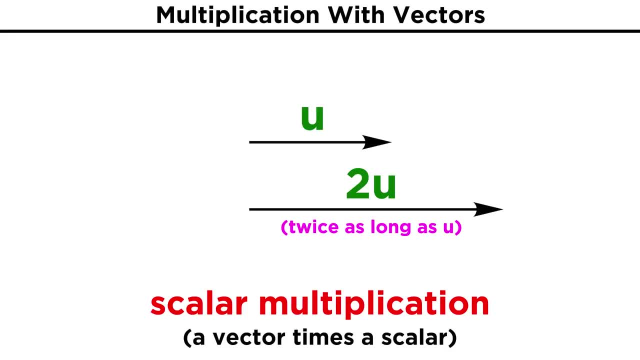 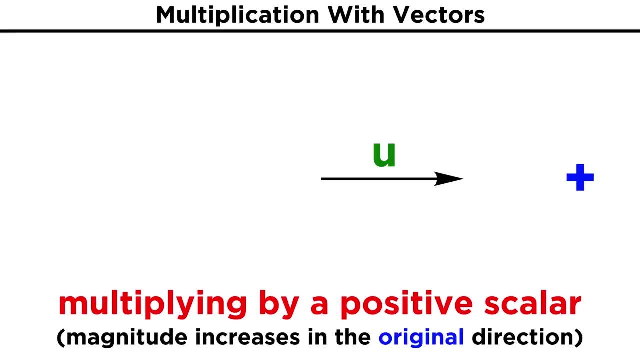 the length of the vector, making it start from the same point but reach twice as far in the direction it is pointing. So when multiplying a vector by a scalar that is greater than zero, we just multiply the length of the vector by the scalar. 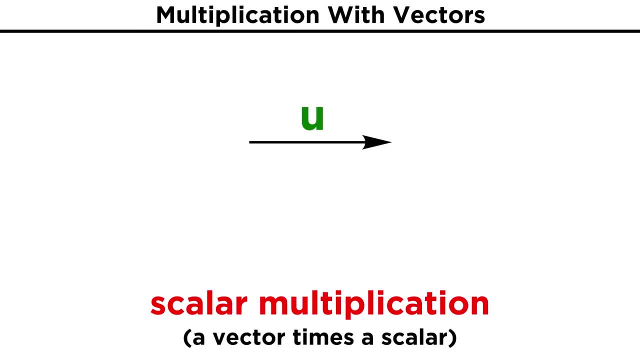 addition, geometrically We can also perform multiplication with vectors. The simplest way to do this is called scalar multiplication. This is when a vector is multiplied by a scalar, which is just a number. So if we have some vector u and we multiply it by the scalar two, all we do is double. 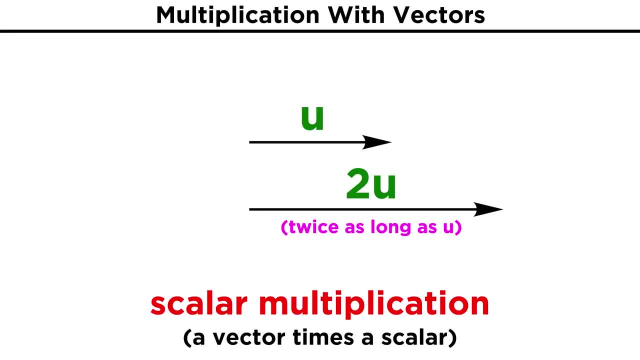 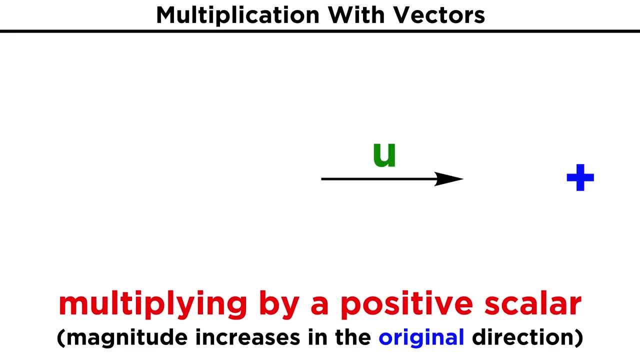 the length of the vector, making it start from the same point but reach twice as far in the direction it is pointing. So when multiplying a vector by a scalar that is greater than zero, we just multiply the length of the vector by the scalar. 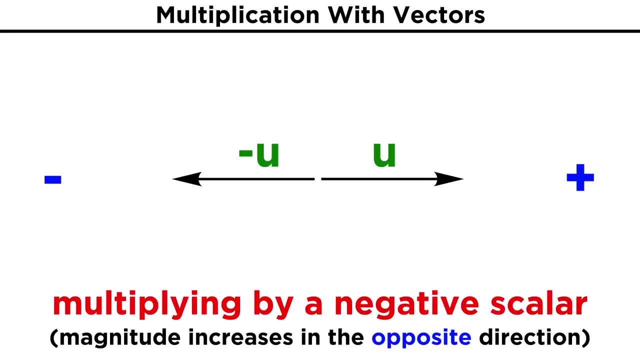 If the scalar is less than zero or a negative number, we still alter the length of the vector in the same way, but we also reorient it to point in the negative direction relative to its original position, which is just precisely the opposite direction, or 180 degrees away. 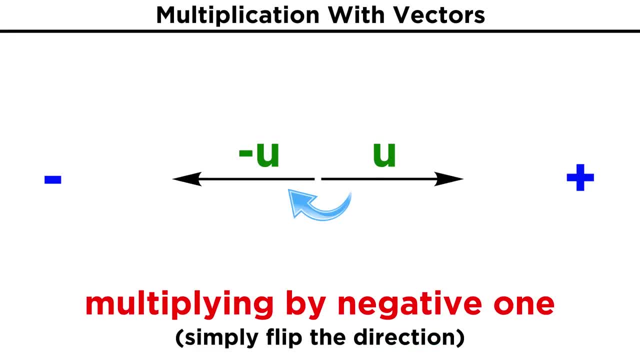 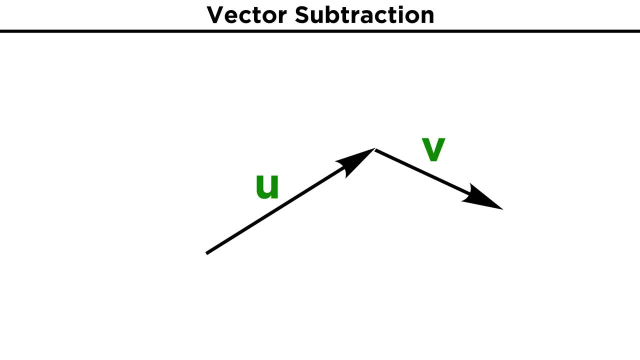 So vector u times the scalar negative one will just flip it over in this manner to give us negative u. This understanding will allow us to now perform vector subtraction. If we have two vectors, u and v, aligned as we did previously, how can we get u minus? 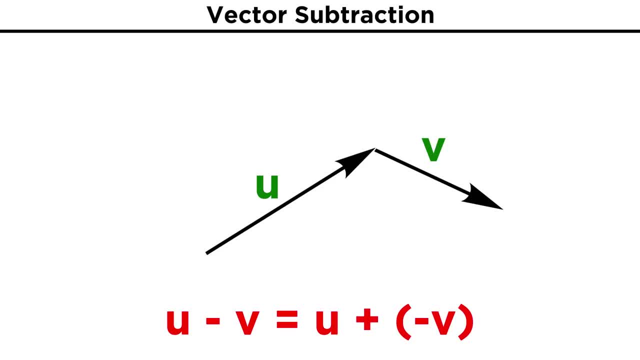 v. Well, u minus v is the same thing as u plus negative v. So if we take v and flip the direction, it is now negative v and we can just do the vector addition, like we already learned. Completing the triangle with u and negative v will give us u plus negative v or u minus. 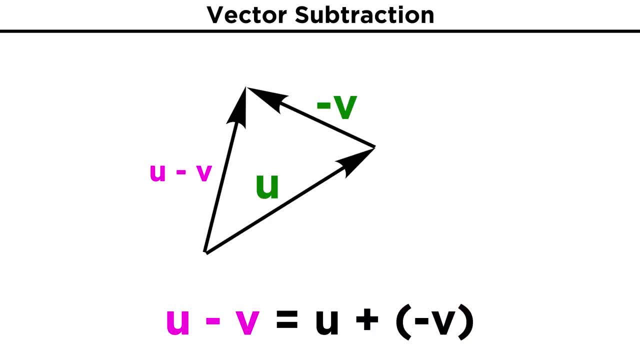 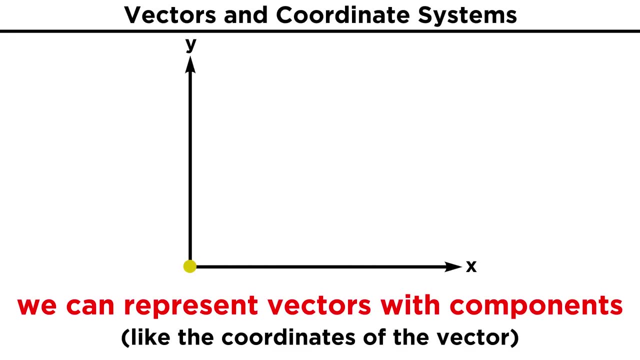 v and we have just performed vector subtraction. We can combine scalar multiplication and vector addition and subtraction to do all kinds of things with vectors which we will see later. We should also note that vectors can be represented by components which are kind of like quarter. 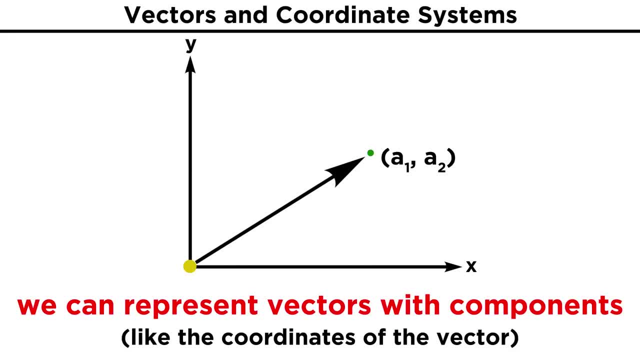 coordinates, Let's say a vector extends from the origin to the point. The vector itself can be represented this way, kind of like the point, but with this bracket-like notation rather than parentheses to distinguish the vector from the ordered pair that represents the point. 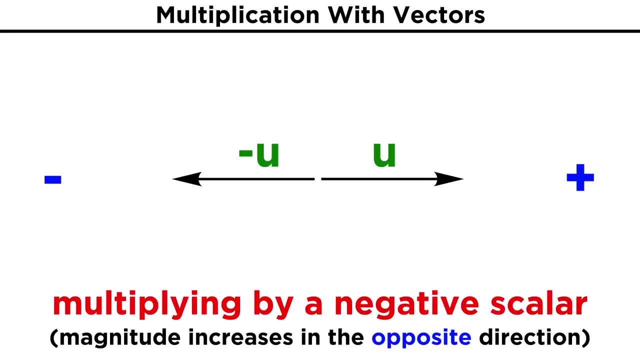 If the scalar is less than zero or a negative number, we still alter the length of the vector in the same way, but we also reorient it to point in the negative direction relative to its original position, which is just precisely the opposite direction, or 180 degrees away. 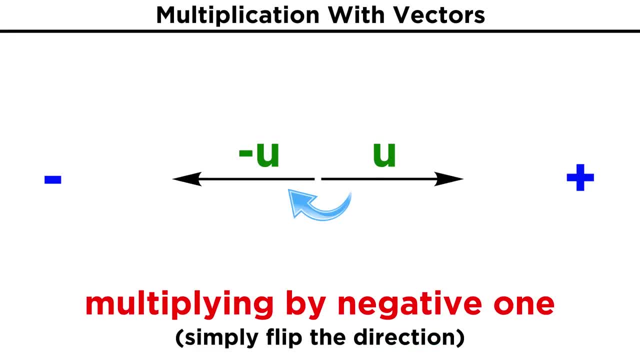 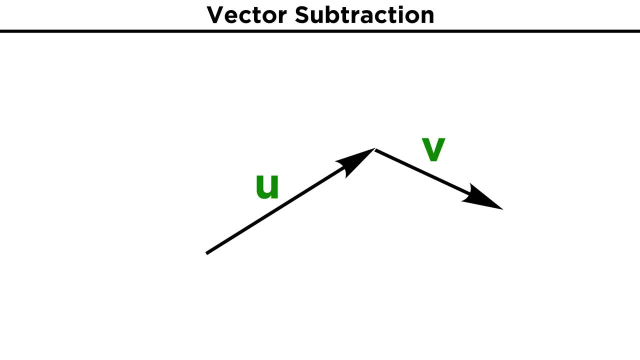 So vector u times the scalar negative one will just flip it over in this manner to give us negative u. This understanding will allow us to now perform vector subtraction. If we have two vectors, u and v, aligned as we did previously, how can we get u minus? 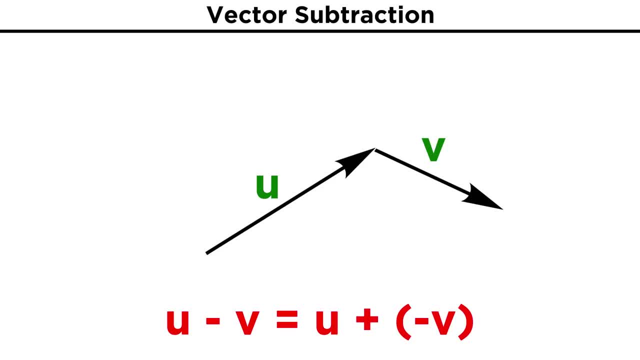 v. Well, u minus v is the same thing as u plus negative v. So if we take v and flip the direction, it is now negative v and we can just do the vector addition, like we already learned. Completing the triangle with u and negative v will give us u plus negative v or u minus. 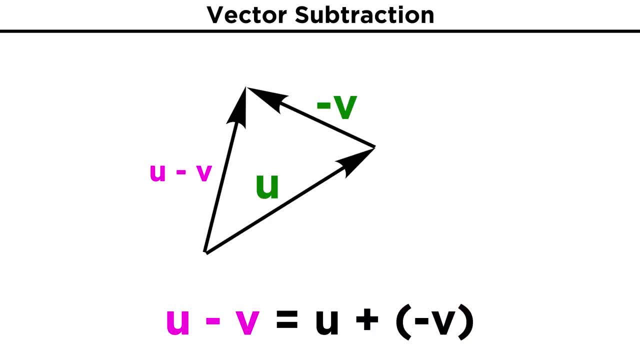 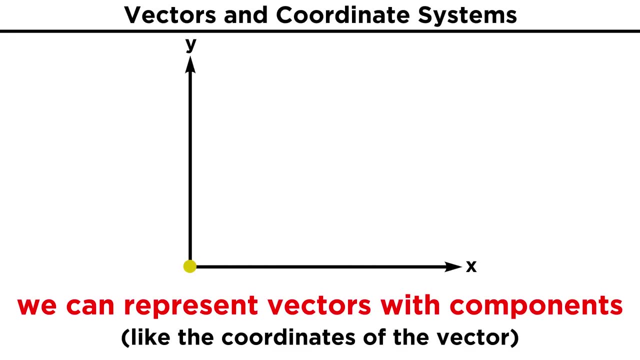 v and we have just performed vector subtraction. We can combine scalar multiplication and vector addition and subtraction to do all kinds of things with vectors which we will see later. We should also note that vectors can be represented by components which are kind of like quarter. 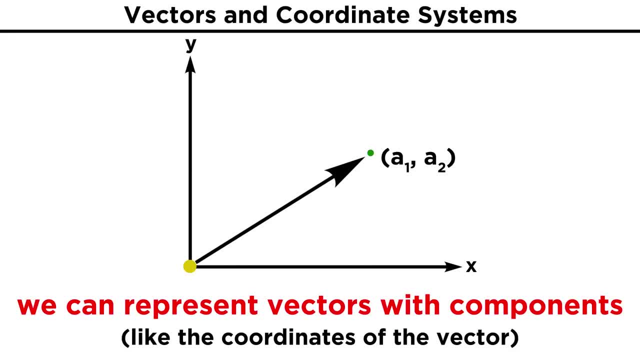 coordinates, Let's say a vector extends from the origin to the point. The vector itself can be represented this way, kind of like the point, but with this bracket-like notation rather than parentheses to distinguish the vector from the ordered pair that represents the point. 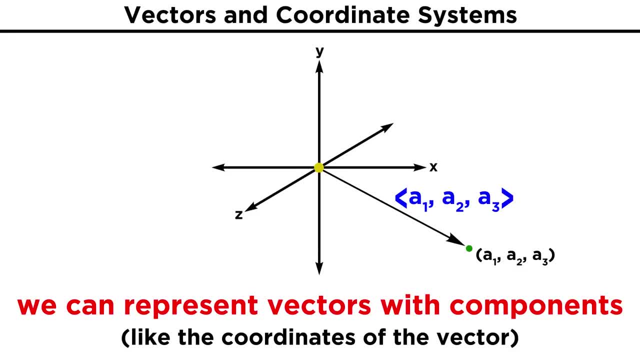 This can be done in a three-dimensional coordinate system as well, with x, y and z axes. The length of the vector can be divided by the order of the vector. This can be done in a three-dimensional coordinate system as well, with x, y and z axes. 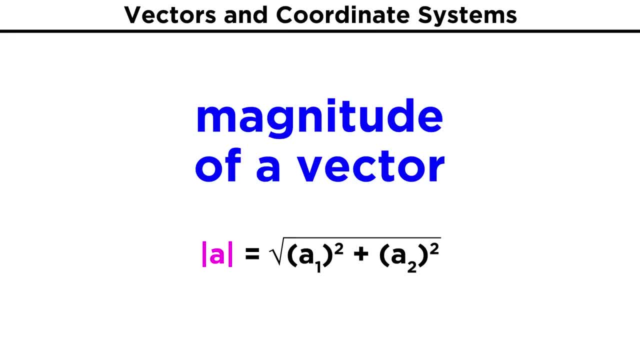 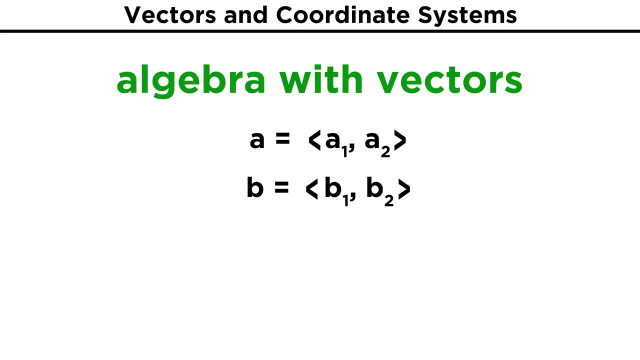 The length or magnitude of a vector represented by these brackets here that look like absolute value brackets can be calculated by finding the square root of the sum of the squares of its components. We can also use this information to do more algebra with vectors. If we have a vector A with components A one and A two and another vector B with components. B one and B two. the sum of these vectors, or A plus B, will have a size of x and c and a square root of 1, and means that we've WordPress. prefer a or b. the sum of them is a plus b. 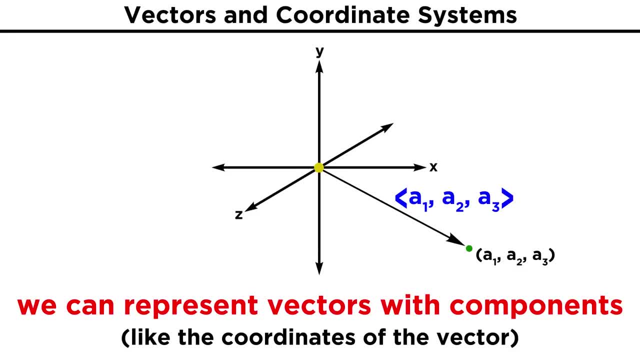 This can be done in a three-dimensional coordinate system as well, with x, y and z axes. The length of the vector can be divided by the order of the vector. This can be done in a three-dimensional coordinate system as well, with x, y and z axes. 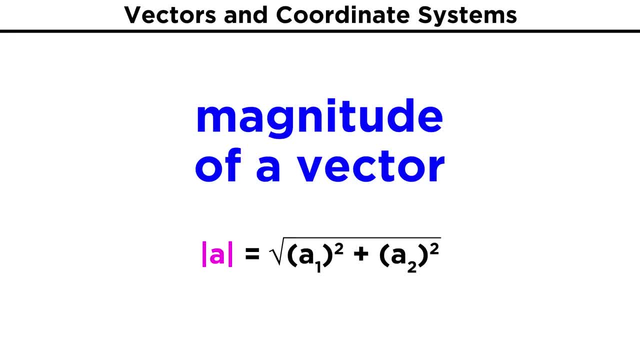 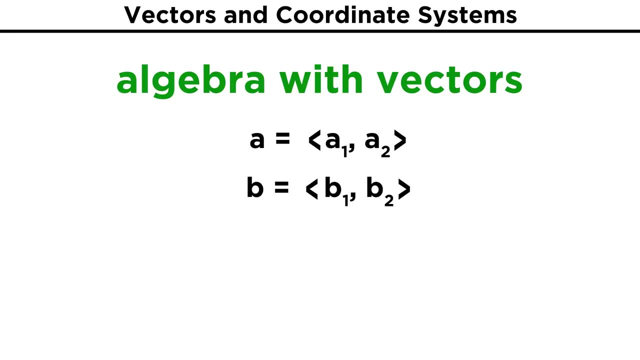 The length or magnitude of a vector represented by these brackets here that look like absolute value brackets can be calculated by finding the square root of the sum of the squares of its components. We can also use this information to do more algebra with vectors. If we have a vector A with components A1 and A2, and another vector B with components B1. 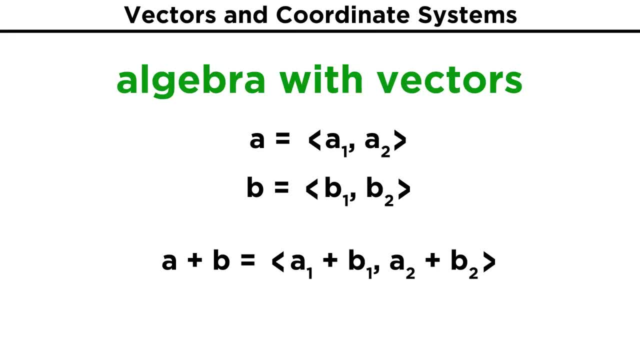 and B2, the sum of these vectors, or A plus B, will have the same number of vectors as the components A1 plus B1 and A2 plus B2. The same can be said for vector subtraction: we just subtract the corresponding components. 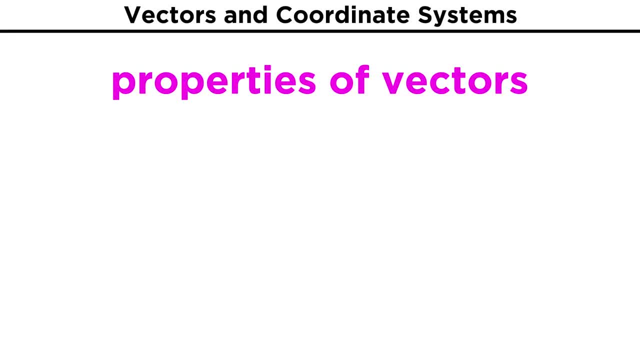 In fact, let's quickly mention some important properties of vectors. The commutative and associative properties of addition apply to vectors like the way that A plus B equals B plus A and the way that A plus the quantity B plus C equals the quantity A plus B plus A. 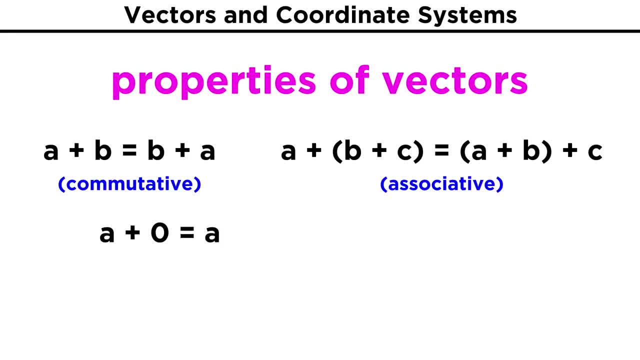 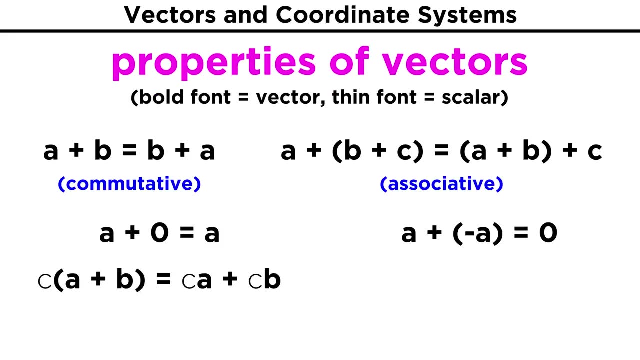 Any vector plus the zero vector, which is the vector with zeros for all its components, will simply give the same vector we started with. Any vector plus the negative version of that same vector, which is simply a vector minus itself, is the zero vector. 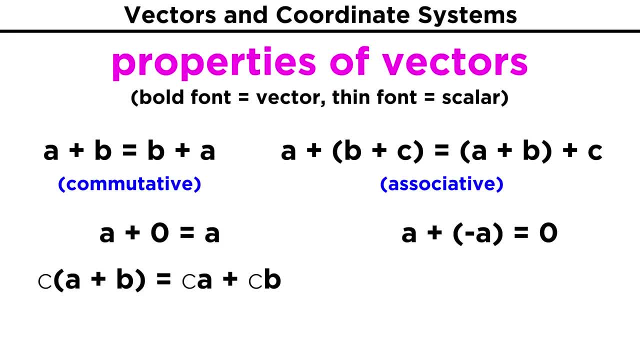 While we can't add a vector and a scalar. a scalar can be distributed across a sum of vectors and a vector can be distributed across a sum of scalars. A product of A, The product of A, The product of B, The product of C. 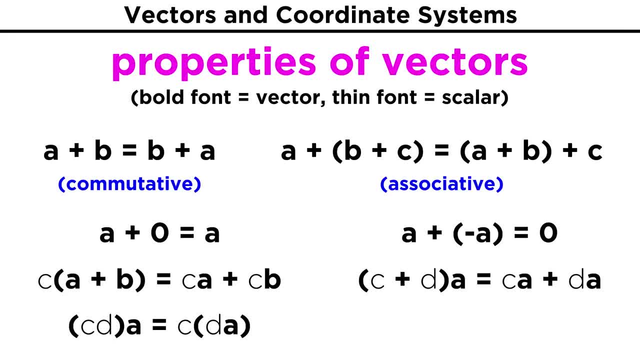 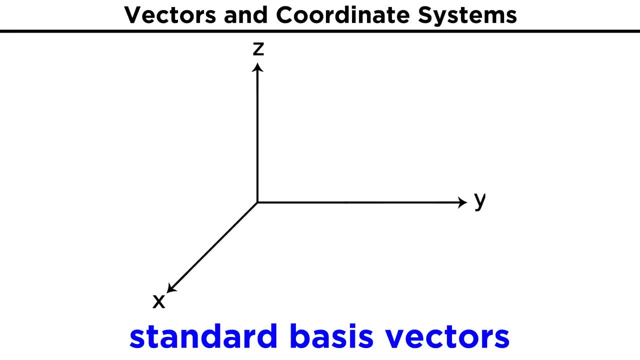 The product of D. And now let's think about some more simple ways to know vector subtraction. There is one other way we can represent vectors that will be important to know, and it involves standard basis vectors, which are unit vectors, meaning they have a length of one. 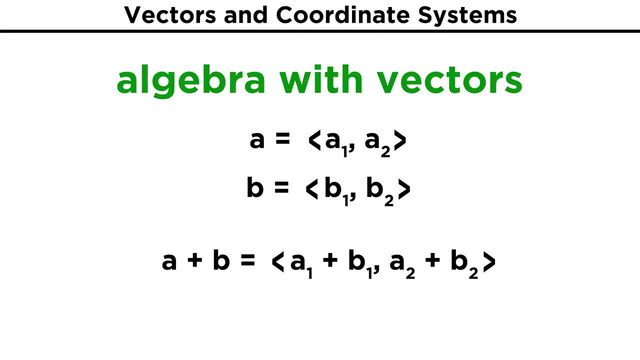 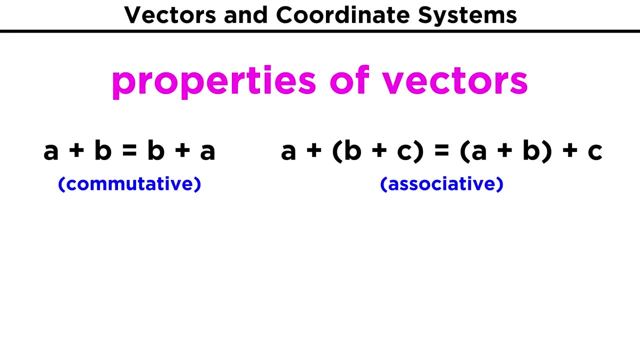 have the components a1 plus b1 and a2 plus b2.. The same can be said for vector subtraction: we just subtract the corresponding components. In fact, let's quickly mention some important properties of vectors. The commutative and associative properties of addition apply to vectors like the way: 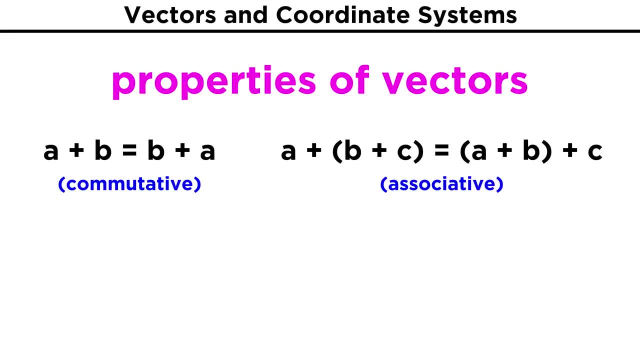 that a plus b equals b plus a, and the way that a plus the quantity b plus c equals the quantity a plus b plus c, Any vector plus the zero vector, which is the vector with zeros for all its components, will simply give the same vector we started with. 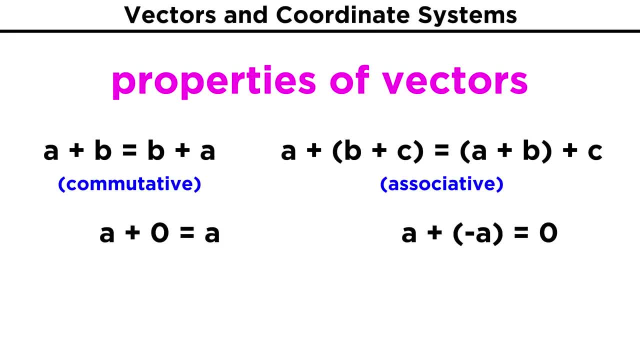 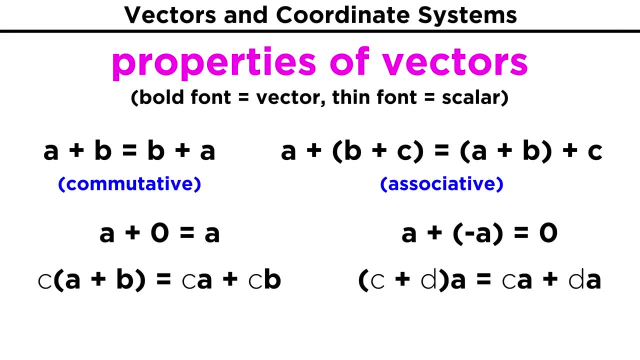 Any vector plus, the negative version of that same vector, which is simply a vector minus itself, is the zero vector. While we can't add a vector and a scalar, a scalar can be distributed across a sum of vectors and a vector can be distributed across a sum of scalars. 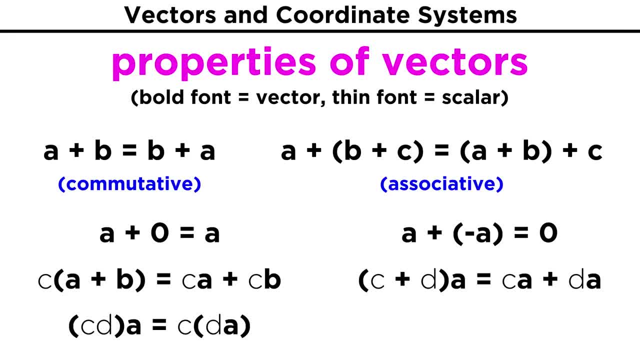 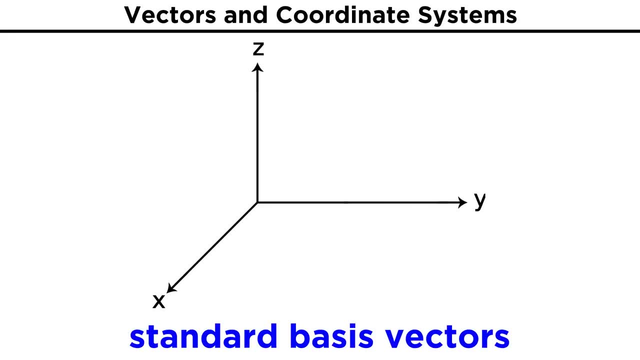 A product of scalars times, a vector is the same as one of the scalars times the product of the other scalar and the vector, And one times any vector is simply that vector. Those are the important properties we should understand. There is one other way we can represent vectors that will be important to know, and it involves 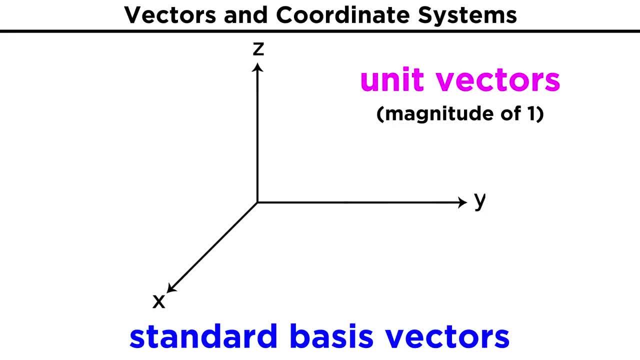 standard basis vectors, which are unit vectors, meaning they have a length of one. If we are in a three-dimensional coordinate system, any vector can be represented by three components. The vector with the components one, zero, zero, extending one unit along the x-axis is: 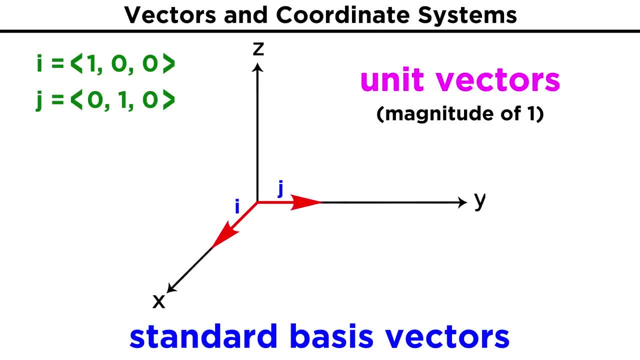 denoted by a lowercase i. The vector with components zero. one. zero extending one unit along the y-axis is denoted by a lowercase j and zero. zero one extending one unit along the z-axis is denoted by a lowercase j. 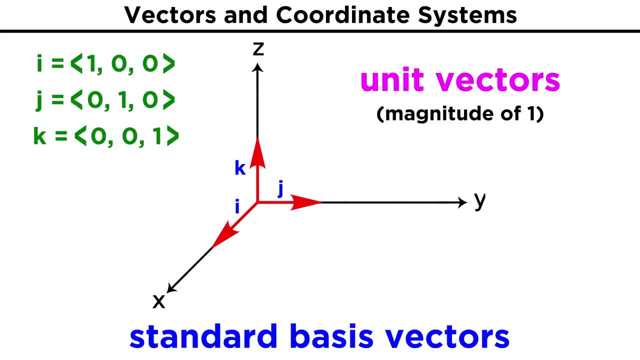 We can now represent any vector with multiples of i, j and k. So five negative two nine can also be five i minus two j plus nine k. This also works in two dimensions. we just lose the k. The reason this is useful is that algebraic manipulations can become much more intuitive. 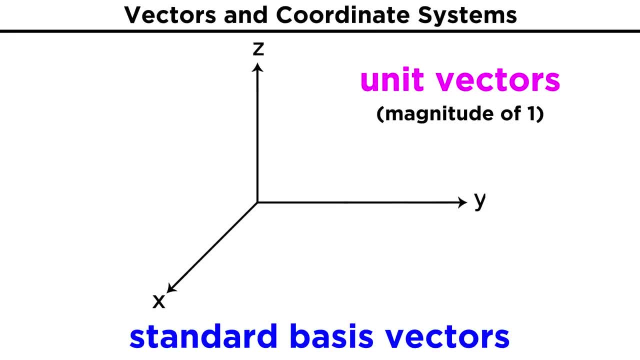 If we are in a three-dimensional coordinate system, Any vector can be represented by three components. The vector with the components one, zero, zero, extending one unit along the X axis is denoted by a lowercase I. The vector with components zero- one, zero- extending one unit along the Y axis is denoted. 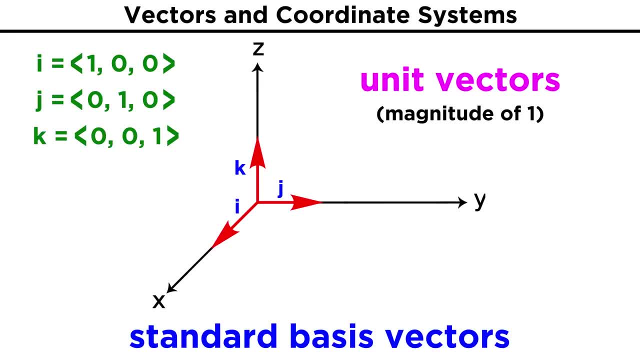 by a lowercase J and zero, zero one. extending one unit along the Z axis is denoted by a lowercase K. We can now represent any vector with multiples of I, J and K. so five negative two nine can also be five. I minus two J plus nine K. 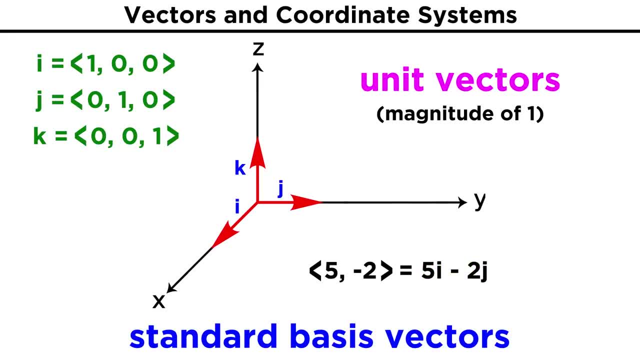 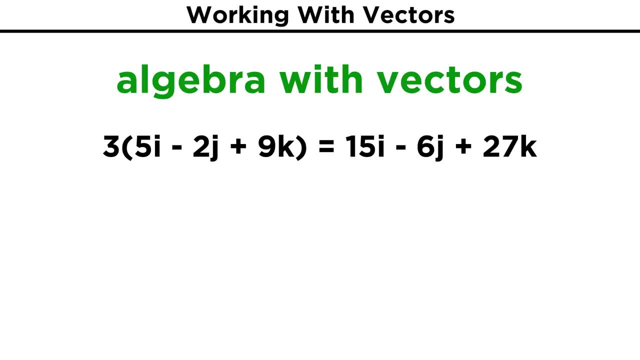 This also works in two dimensions. we just lose the K. The reason this is useful is that algebraic manipulations can become much more intuitive, as operations like multiplying a vector by a scalar are reduced to simply distributing a number across the vector. We can also add two vectors together without having to draw them. 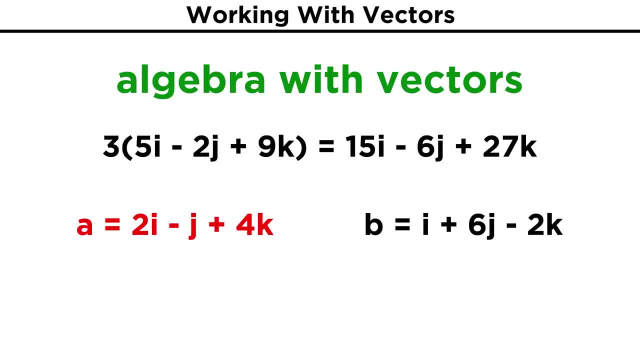 We can simply define one vector A which we can say is equal to two I minus J plus four K, and another vector B which is I plus six J minus two K. Then, to do something like two A plus three B, we can simply change A and B to this other. 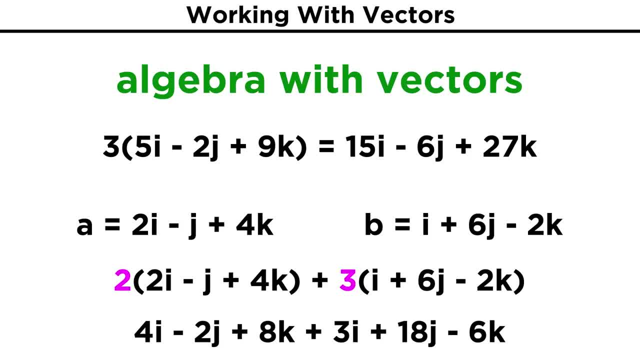 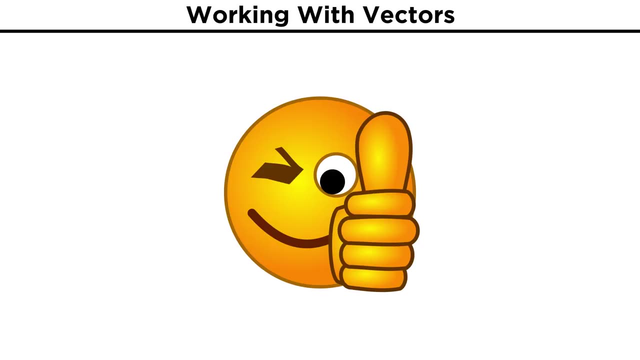 notation. We can also add a scalar across the sum it operates on. Then we simply combine like terms and we end up with seven I plus sixteen J plus two K, and we have performed this complex operation using simple algebra. Now that we know how to perform a few different operations with vectors, let's check comprehension. 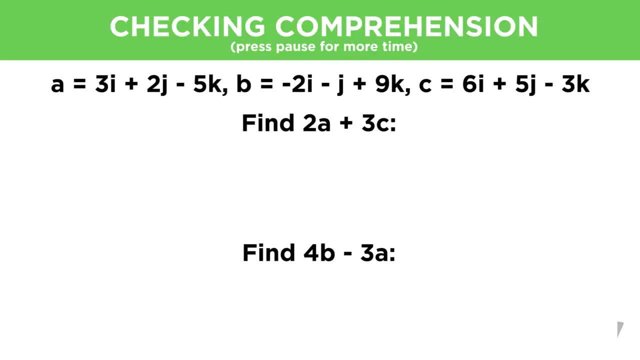 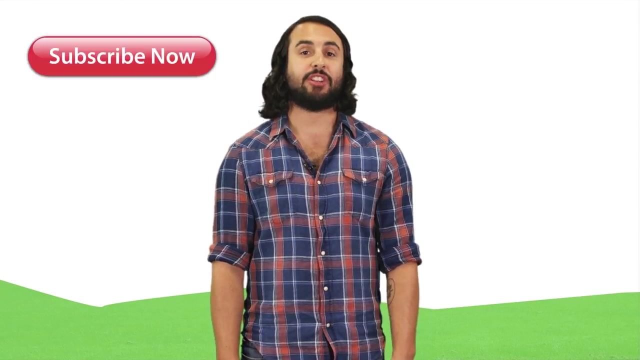 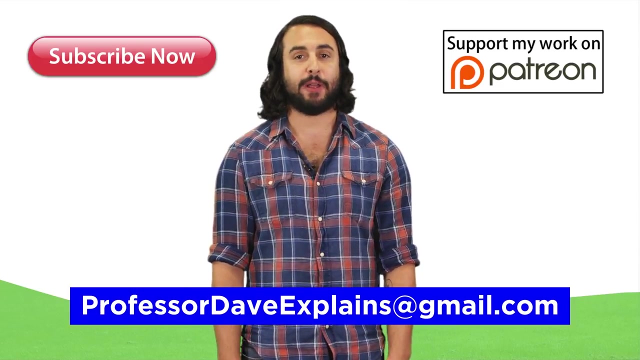 Thanks for watching guys. Subscribe to my channel for more tutorials. support me on Patreon so I can keep making content And, as always, feel free to email me professordaveexplains at gmail dot com.